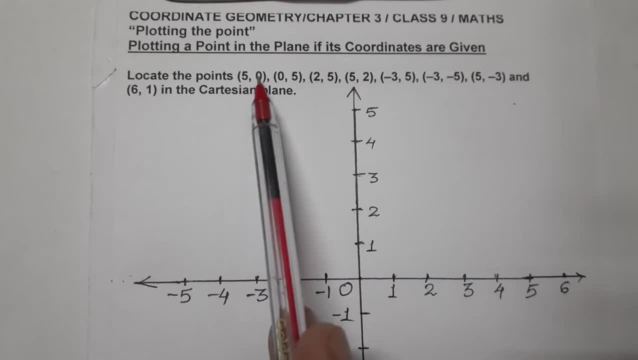 You know this is Cartesian plane. First point is 5, 0.. Children, if the y coordinate is 0, then that point will lie on x axis. So 5, 0.. So we have to move from origin 5 distance, 5 points away from the origin. 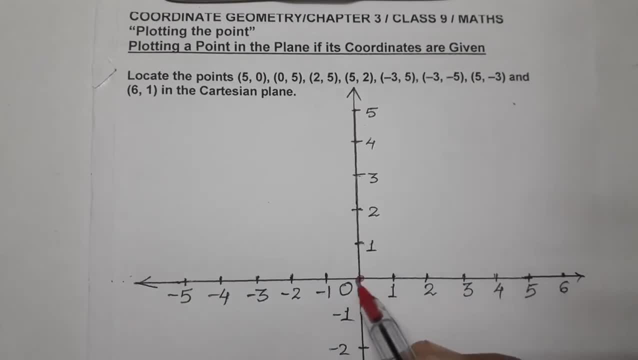 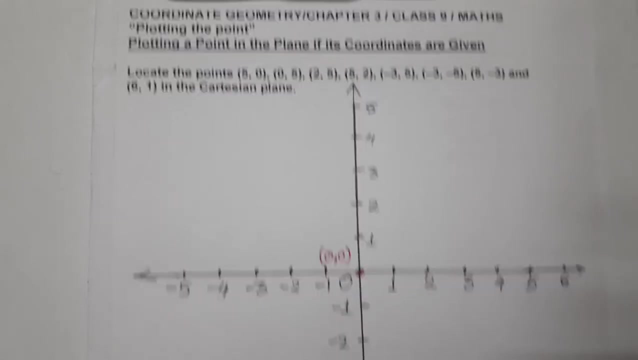 Okay, so let's start. This is our origin. This Cartesian coordinate is 0, 0.. And from here we have to move 5 points towards the positive x axis. This is positive x axis. this is negative x axis. this is positive y axis. this is negative y axis. this one, this one is negative y x, this one in. 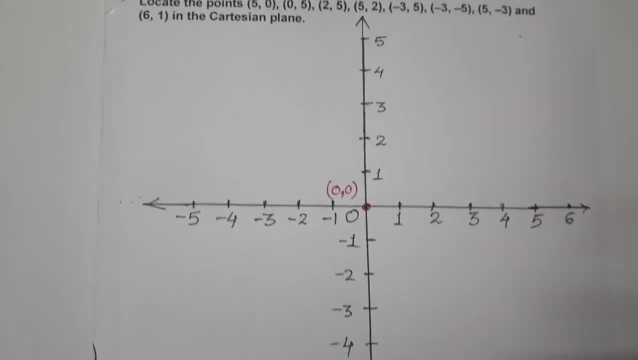 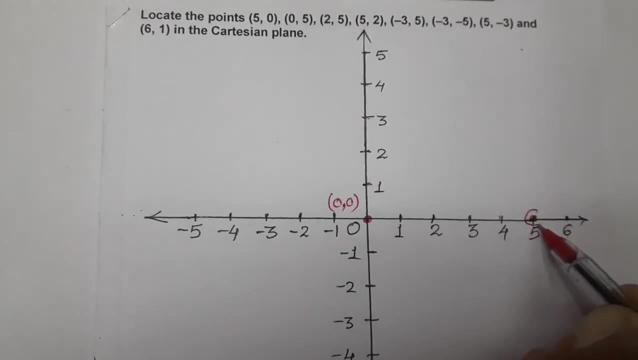 negative y axis. now what, uh? what is our point? first, five zero. so x is five, means this is the point and y will not move because the y coordinate is zero and y coordinate there. then we have to move towards up or down according to the point. so first point is five zero. we have plotted. 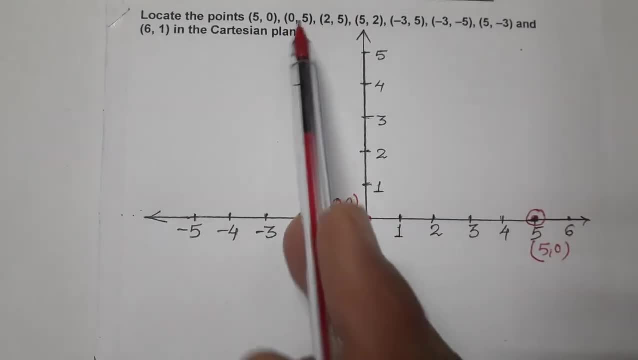 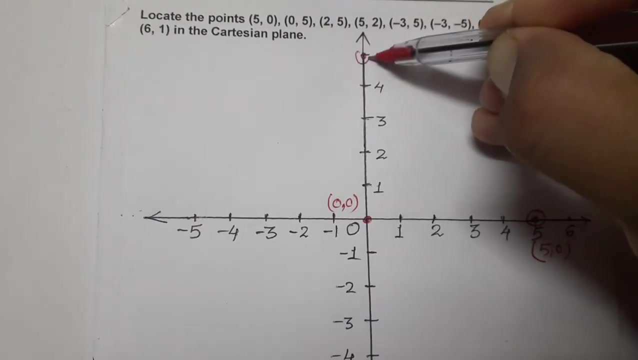 now see the second point: zero, five. so here x coordinate is zero, and whenever x coordinate is zero, the point will lie on y axis. so zero, five, zero and five, so five will come here. five points plus five is there, so five points towards up. so this is zero, five. 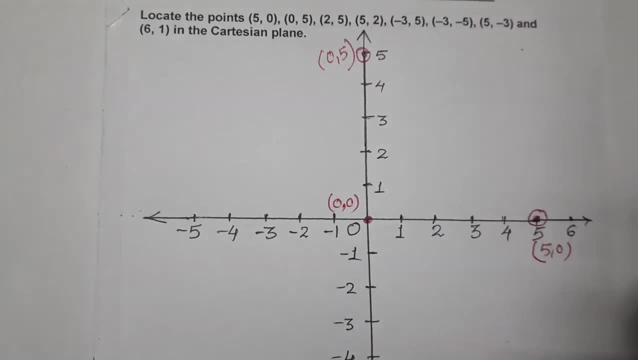 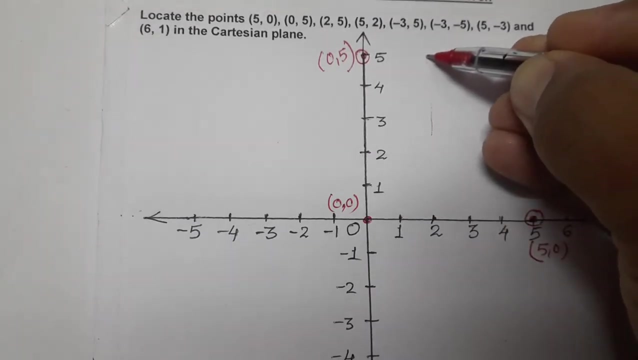 now the third. one is two. five means first of all we have to move towards, uh, positive x, this is two points, one, two. here. then we have to move towards up five points, so two and this is five, this is two, five, x is two, y is five. 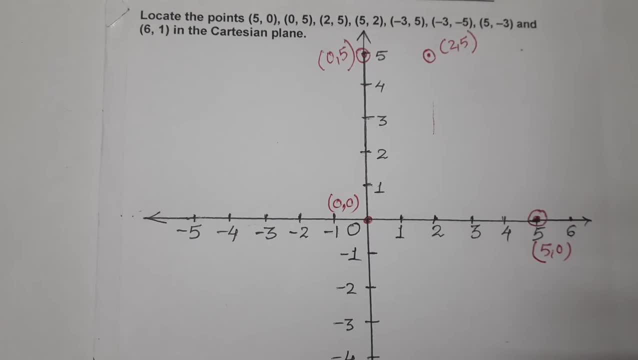 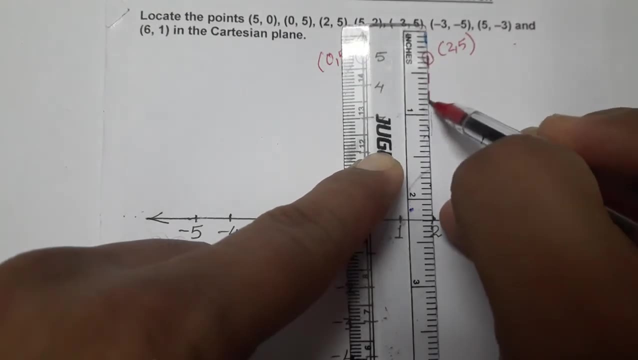 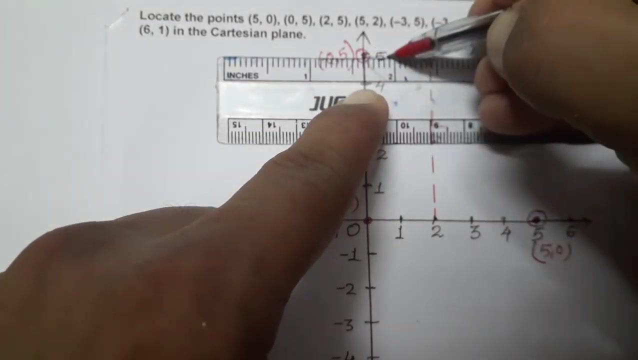 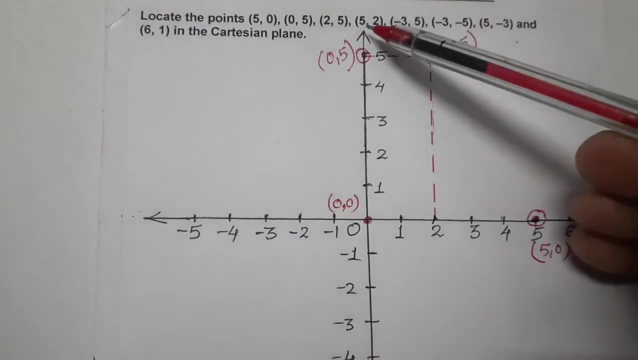 the next point, and you can draw lines also. if you wish, you can draw lines. it is not graph, so you can make lines. you can draw lines like this, as it is not a graph paper. okay, now the next one is five, two, five. where is five? five is here. x coordinate five. and now we have to move two points towards y axis. 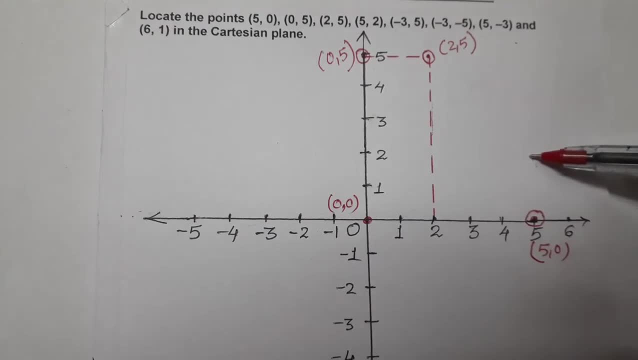 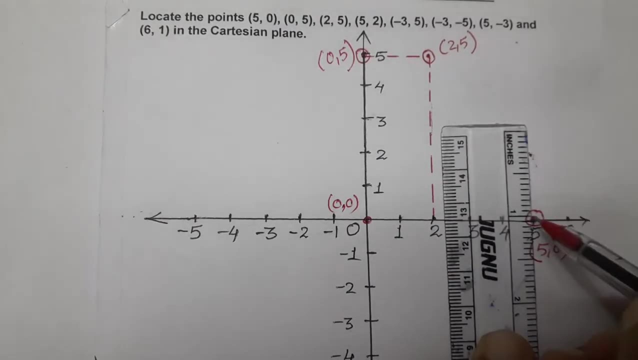 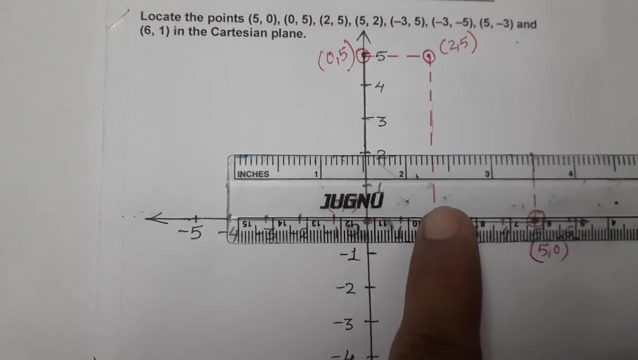 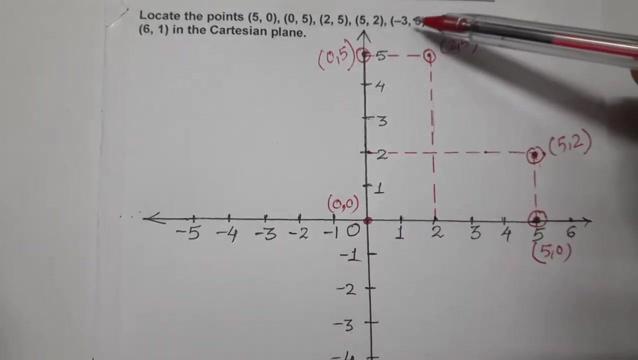 that is here. so the point is will be here. now make line, dotted lines. so this is five, two. this point is five, two. now see the next point. next point is minus three, five. now we have to move towards negative x axis minus three. so where is minus three? one, two, three: this is minus three. 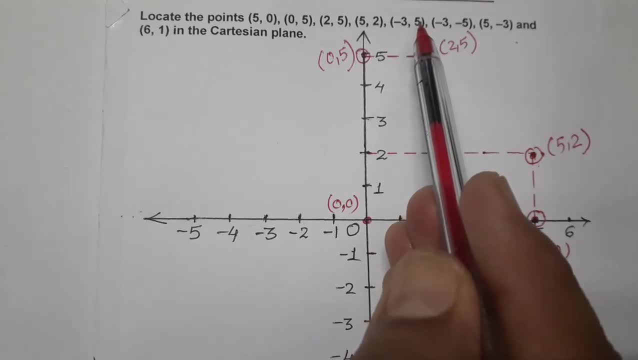 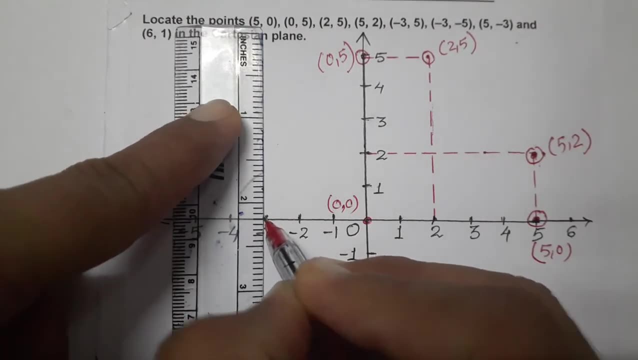 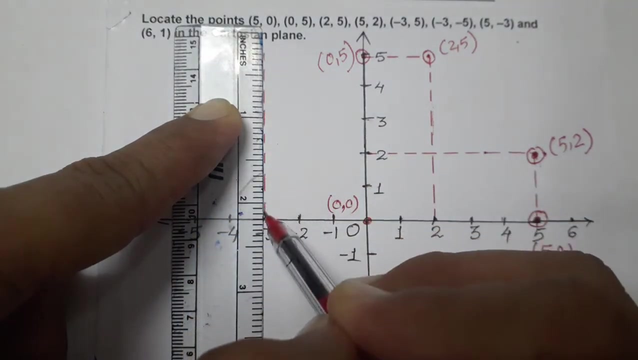 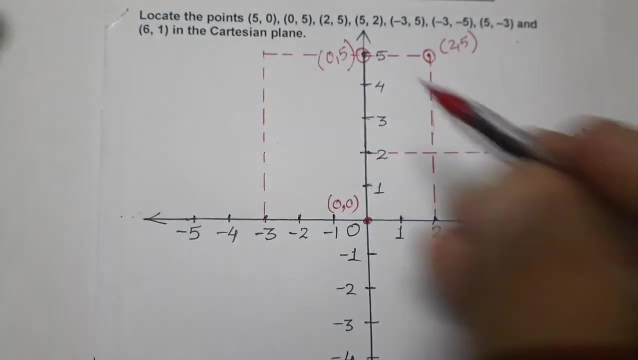 now see 5 minus 3, 5, 5. positive y axis: minus 3 to 5. 5 is where here, so minus 3, 5. 5 is here, minus 3, now 5. okay, so this point is come to be known as minus 3- 5. 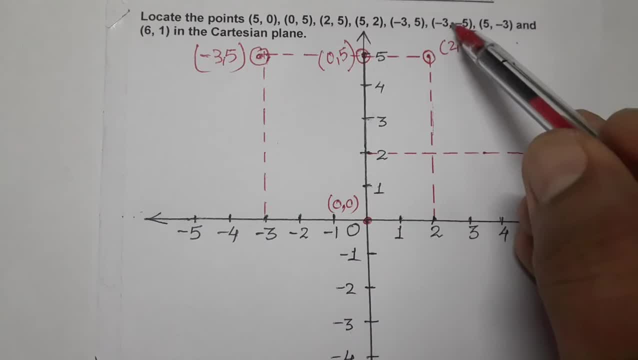 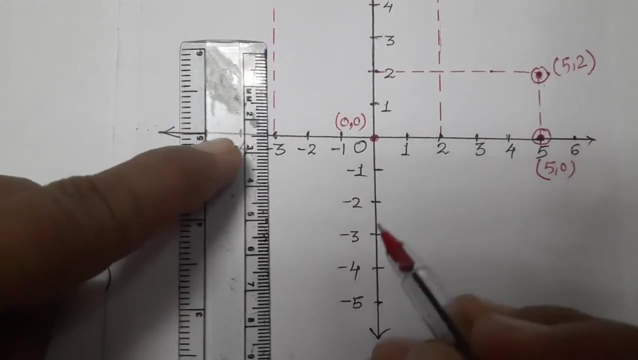 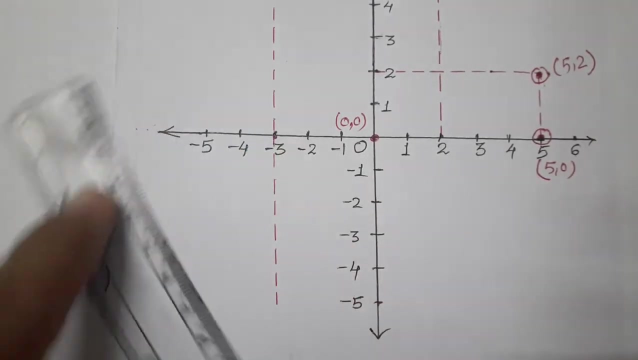 next point is minus 3 minus 5. first negative x axis, minus 3 here and minus 5 negative y axis. we have to move towards down, minus 5. so here minus 5. so first let's move. so this is minus 3 over now. this is minus 5. 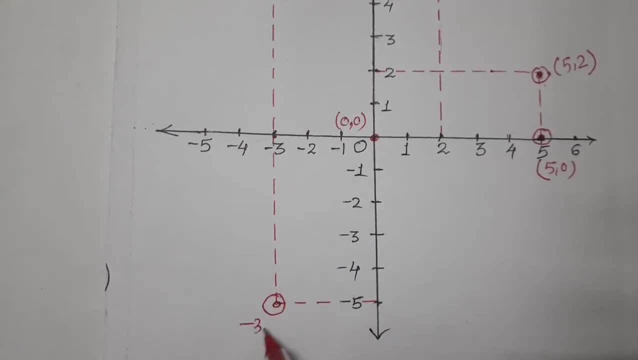 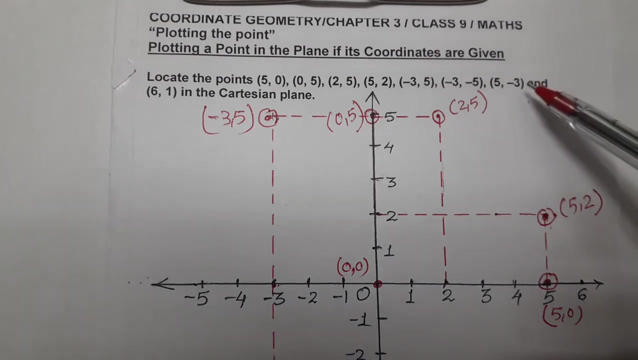 so this one is minus 3 minus 5. x coordinate minus 3, y coordinate: how much minus 5. and next one see children. next one is 5 minus 3.. x-axis 5: y-axis minus 3, 5, so say 5 where 5, 5 is here. 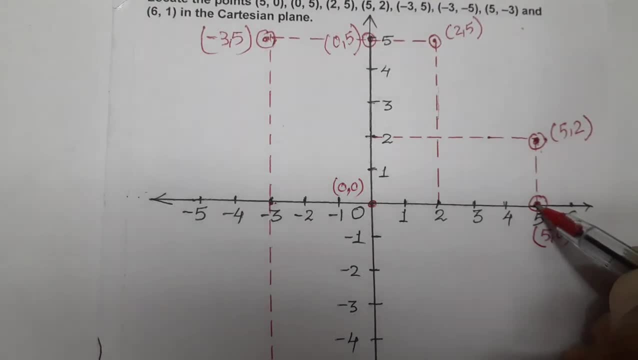 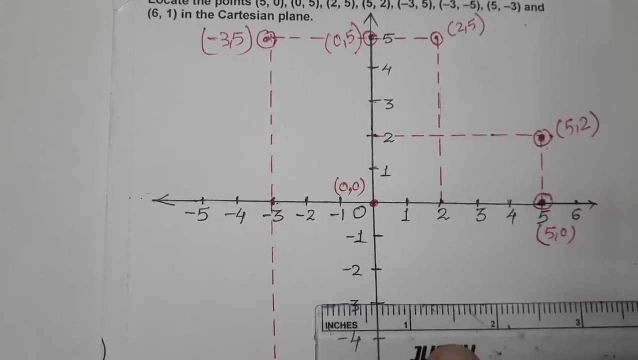 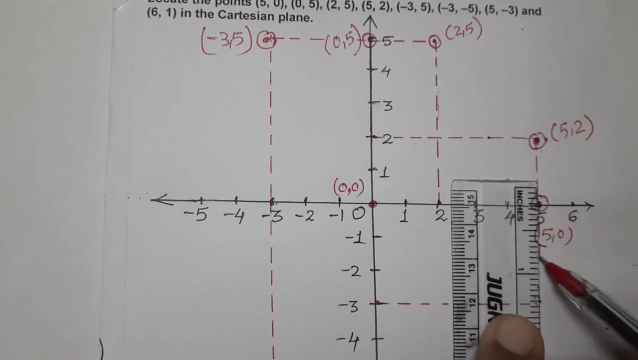 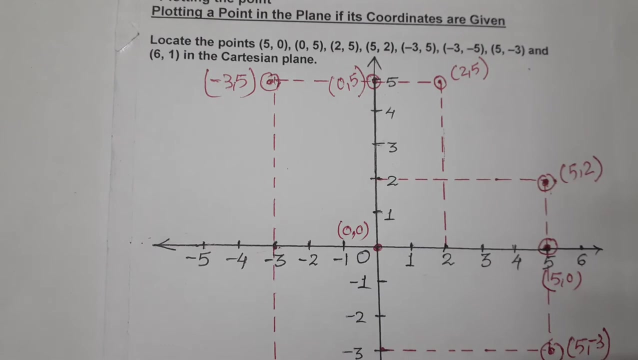 this is 5 and we have to move towards y-axis minus 3.. So minus 3 is where? Here This is 5 and this is minus 3.. So this point is x coordinate 5, y coordinate minus 3.. Now last one: 6, 1.. x coordinate 6, y coordinate 1..